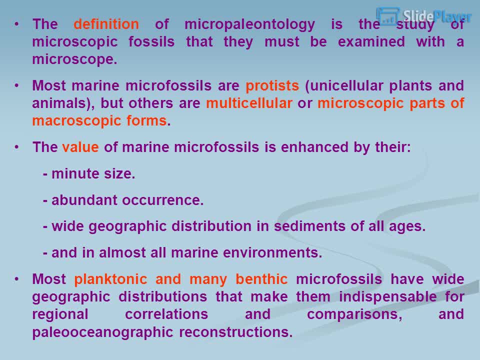 Most marine microfossils are protists, unicellular plants and animals, but others are multicellular, raw, microscopic parts of macroscopic forms. The value of marine microfossils is enhanced by their minute size: abundant occurrence, wide geographic distribution in sediments of all ages. 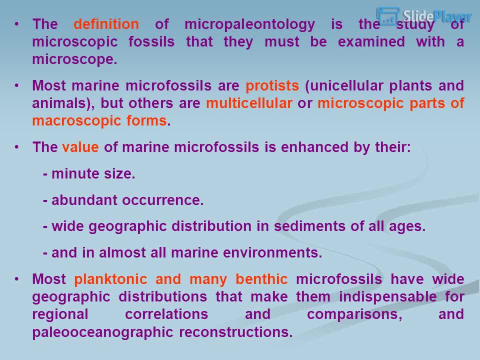 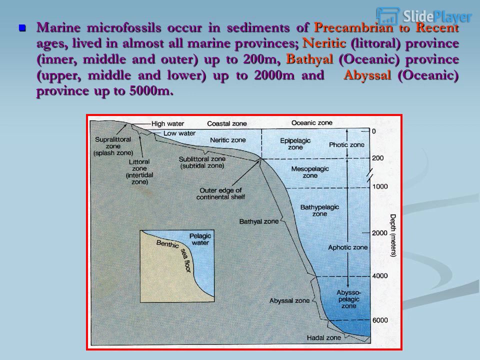 and in almost all marine environments. Most planktonic and many benthic microfossils have wide geographic distributions that make them indispensable for regional correlations and comparisons and paleoceanographic reconstructions. Marine microfossils occur in sediments of pre-Cambrian to recent ages. lived in almost all marine provinces. 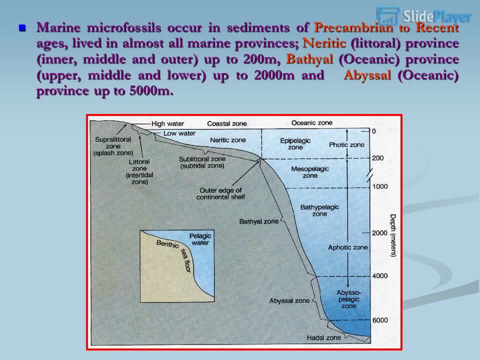 Neuritic Literal Province- Inner, Middle and Outer- up to 200 meters. Bathel Oceania Oceanic Province- Upper, Middle and Lower up to 2,000 meters and Abyssal Oceanic Province up to 5,000 meters. 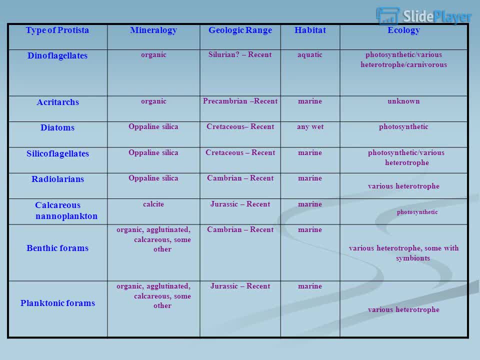 Calcareous nanoplankton: Ecology- Habitat, Geologic range, Mineralogy, Type of protista. Photosynthetic-slash-various heterotrophy-slash-carnivorous Aquatic Synthetic-slash-various heterotrophy-slash-carnivorous Silyurian-dash-recent. 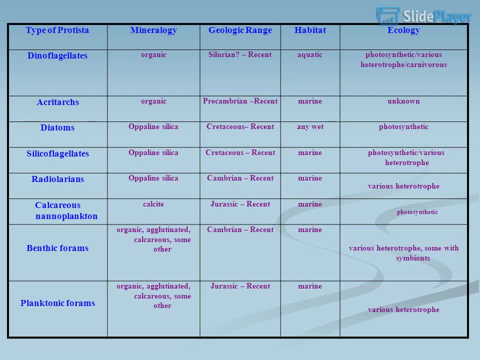 Organic Dinoflagellates: Unknown Marine Pre-Cambrian-recent Acrotarts. Photosynthetic- Any wet Cretaceous-recent Apolline, silica Diatoms. Photosynthetic-slash-various Heterotrophic Heterotrophy Cretaceous-recent. 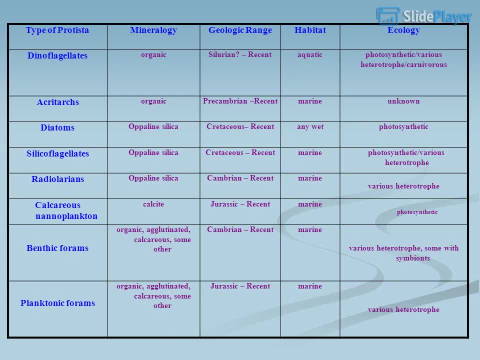 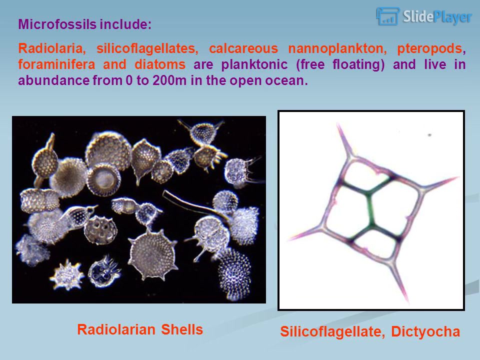 Silicoflagellates: Various heterotrophy Cambrian-recent Radiolarians, Jurassic-recent Calcite, Calcareous. nanoplankton. Various heterotrophy Organic Calcareous. Some other Planktonic-forams Silicoflagellate. 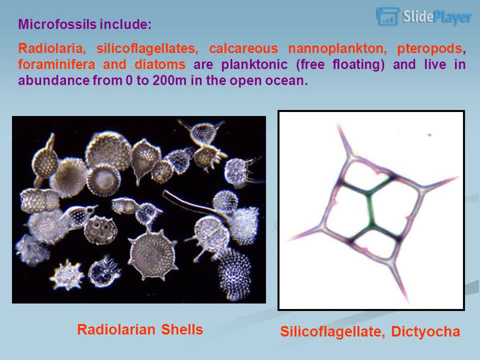 Dictyoca. Microfossils include Radial area Silicoflagellates, calcareous nanoplankton, pteropods, foraminifera and diatoms are planktonic free-floating and live in abundance from 0 to 200 m in the open ocean. 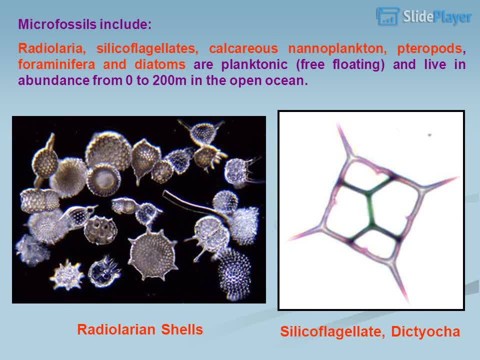 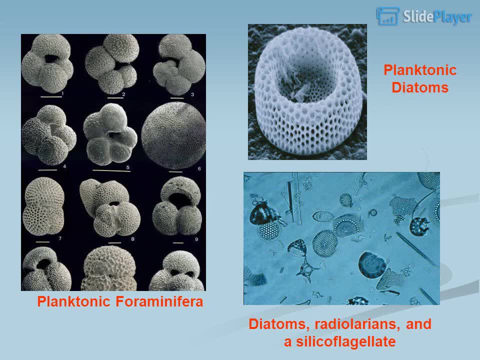 Silicoflagellate Dictyoca Radial area, radiolarian shells, calcareous nanoplankton, pteropods, diatoms radiolarians and planktonic diatoms, planktonic foraminifera diatoms radiolarians and. 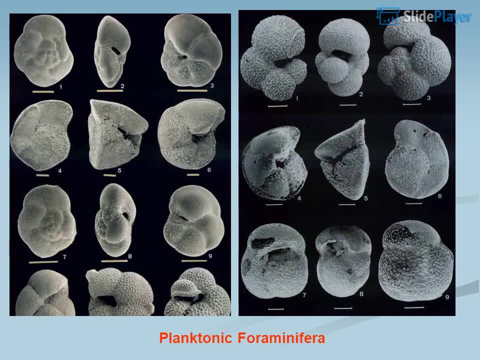 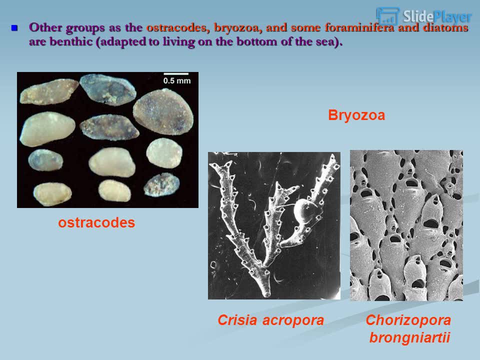 acilicoflagellate, planktonic foraminifera. Other groups as the ostracodes, bryozoa and some foraminifera and diatoms are benthic adapted to living on the bottom of the sea. 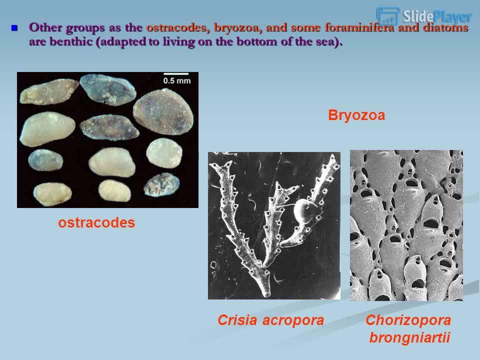 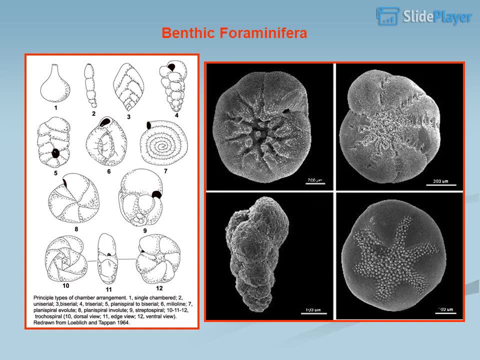 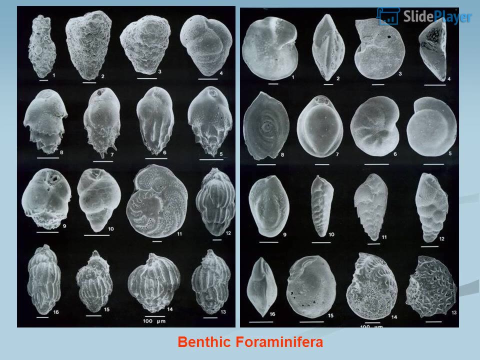 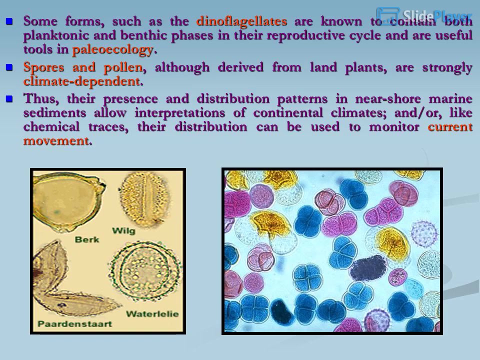 Ostracodes, bryozoa, chrysoacropora, choryzopora, brongnotii, benthic foraminifera and diatoms are benthic foraminifera. Some forms, such as the dinoflagellates, are known to contain both planktonic and benthic. 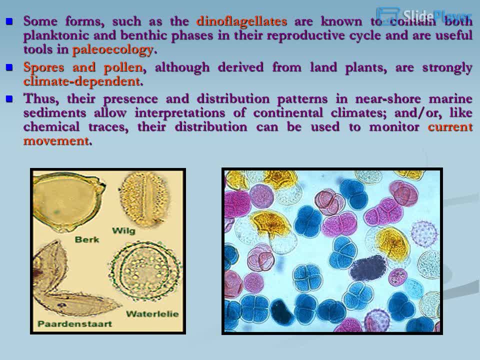 phases in their reproductive cycle and are useful tools in paleoecology. Spores and pollen, although derived from land, plants are strongly climate-dependent. Thus, their presence and distribution patterns in nearshore marine sediments allow interpretations of continental climates and or, like chemical traces, their distribution. 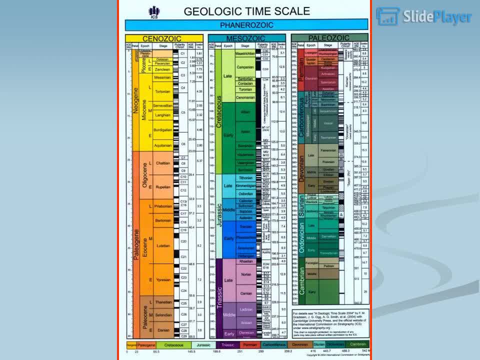 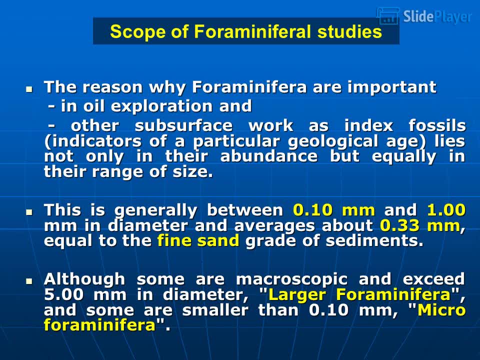 can be used to monitor current movement. Scope of foraminiferal studies. The reason why foraminifera are important In oil exploration and other subsurface work as index fossils indicators of a particular geological age lies not only in their abundance, but equally in their range of size. 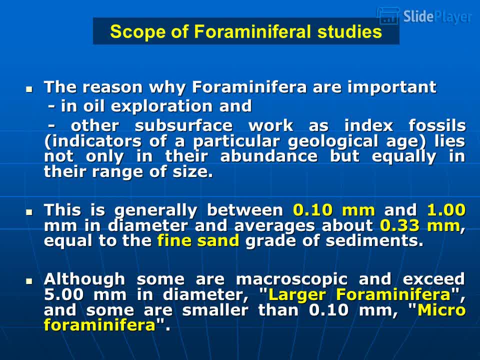 This is generally between 0.10 mm and 1.00 mm in diameter and averages about 0.33 mm, equal to the fine sand grade of sediments. Although some are much more than 0.10 mm in diameter, the average is about 0.33 mm, equal to the fine sand grade of sediments. 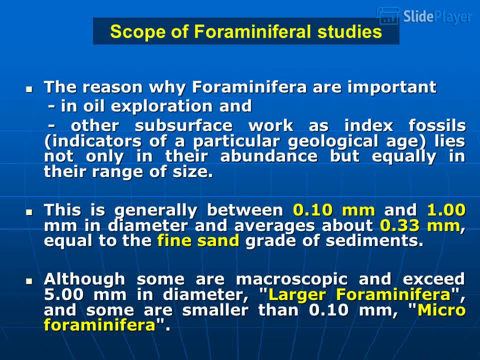 Although some are much more than 0.10 mm in diameter, the average is about 0.33 mm, equal to the fine sand grade of sediments, Although some are macroscopic and exceed 5.00 mm in diameter, larger foraminifera, and some are smaller than 0.10 mm. 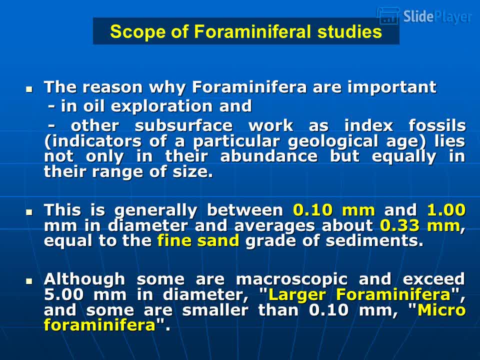 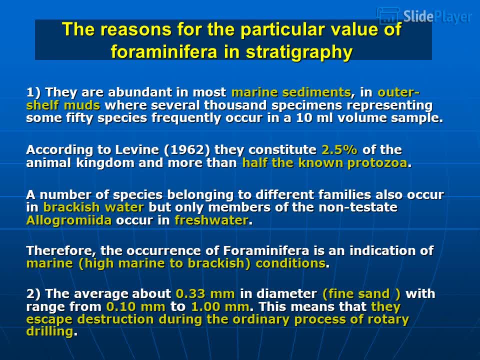 larger foraminifera and some are smaller than 0.10 mm. microforaminifera. The reasons for the particular value of foraminifera in stratigraphy: 1. They are abundant in most marine sediments, in outer shelf muds, where several thousand 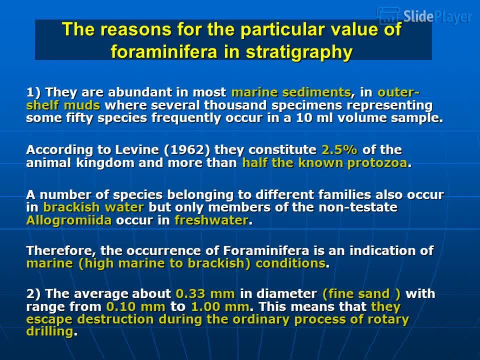 specimens representing some 50 species frequently occur in a 10-mL volume substrate- Genau edible today sample. According to Levine 1962, they constitute 2.5% of the animal kingdom and more than half the known protozoa. A number of species belonging to different families also occur in brackish water. 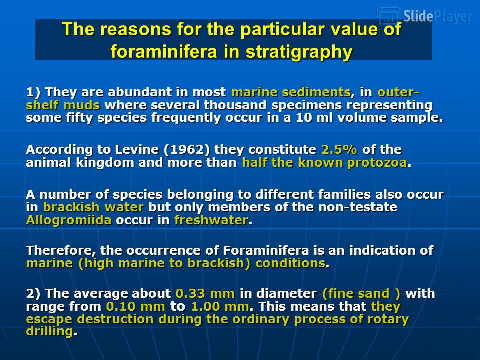 but only members of the non-testate Allogromidae occur in freshwater. Therefore, the occurrence of foraminifera is an indication of marine, high marine to brackish conditions. 2. The average: about 0.33 mm in diameter fine sand with range from 0.10 mm to 1.00 mm. 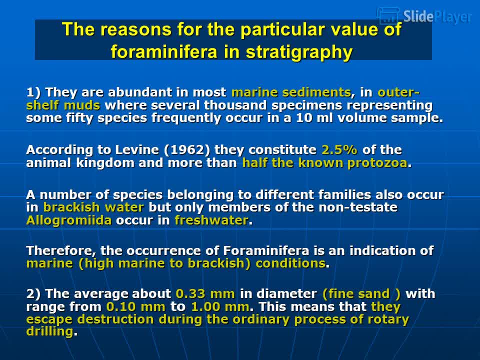 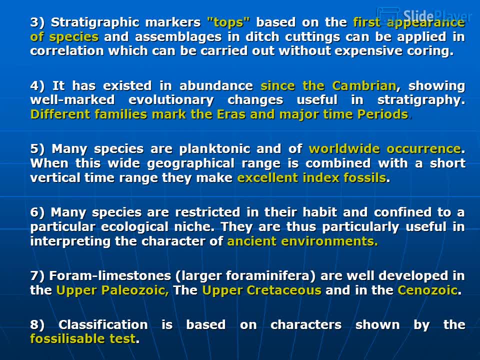 This means that they escape destruction during the ordinary process of rotary drilling. 3. Stratigraphic markers: tops based on the first appearance of species of the same species. These and assemblages in ditch cuttings can be applied in correlation which can be carried out. 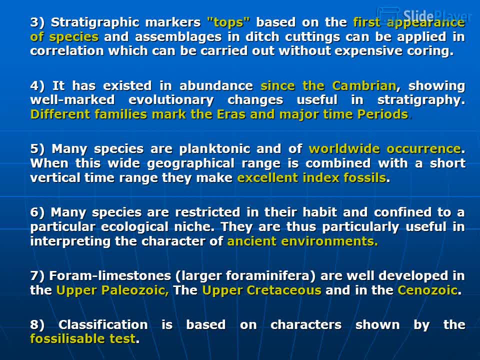 without expensive coring. 4. It has existed in abundance since the Cambrian, showing well-marked evolutionary changes. useful in stratigraphy. Different families mark the eras and major time periods. 5. Many species are planktonic and of worldwide occurrence. When this wide geographical range is,